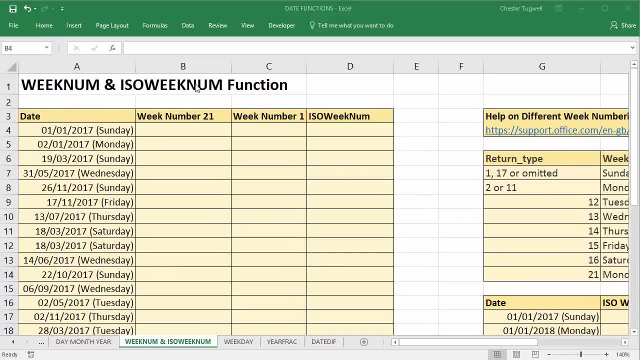 We're going to look at the weeknum and isoweeknum functions. Let's start off with weeknum, and this is going to return the week number for a given date. So if I select that date comma, I then have to specify a return type. So, by and large, this is when your week is going to start. What day of the week is your week going to start? So let's go for 21, Monday and explain a little bit more about return type. 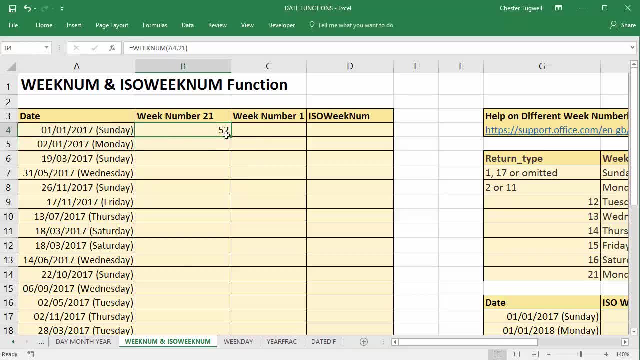 So let's go for 21, Monday and explain a little bit more about return types in a minute. And there we are. If I copy that down, you can see that it's returned the proper week number. Now there's some interesting things going on here. For example, the first of the first 2017 is week 52, and you might think that would be in week 1.. Well, let's try a different return type. Sorry, not weekday, but weeknum. So I take the serial number again and 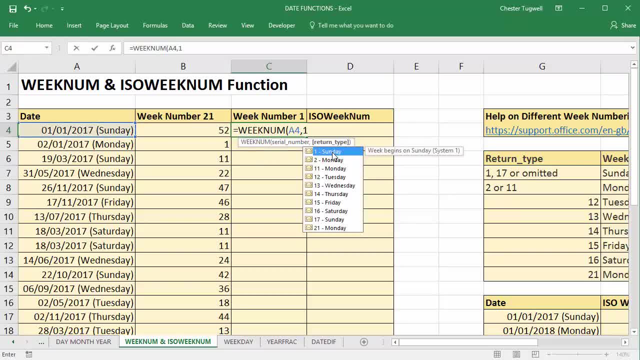 this time I'm going to go for 1 and that has my week starting on a Sunday. And there we are. I copy that down and there we are. Sunday Week starts on Sunday, so we get a return type of 1.. Whereas this here has a return type of 21, which starts the week on a Monday. So you get slightly different results looking down here depending on when your week starts. But when we look at the return types, 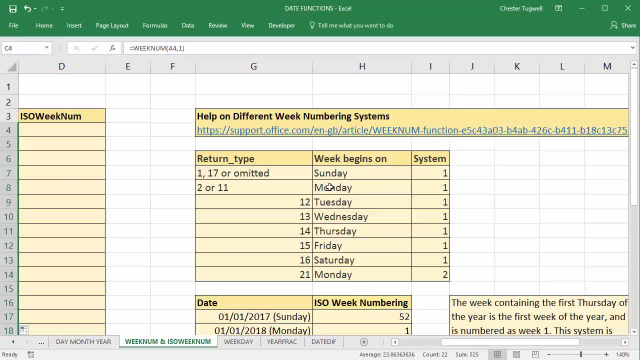 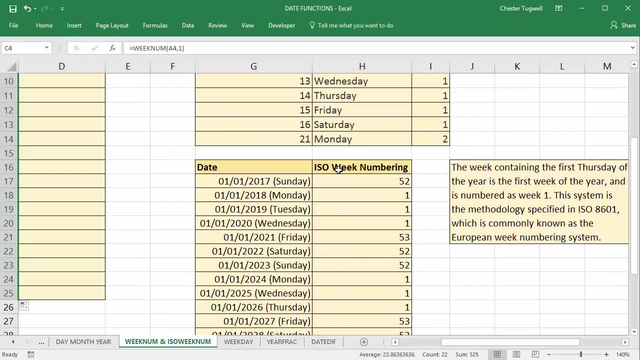 there's actually various Monday options. We had two Mondays in system 1, at the top of the return type list, And then we had a further return type for Monday which was 21.. Now type 21 actually relates to the ISO weeknum function which we'll use over here. 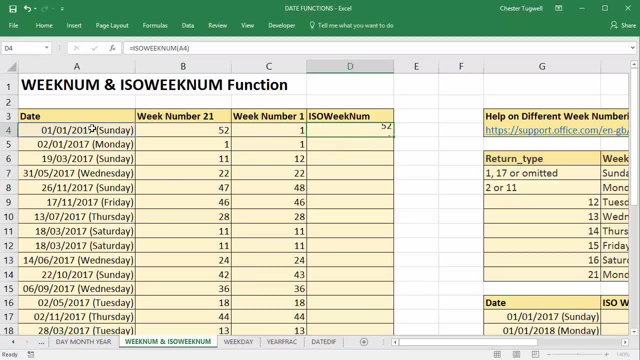 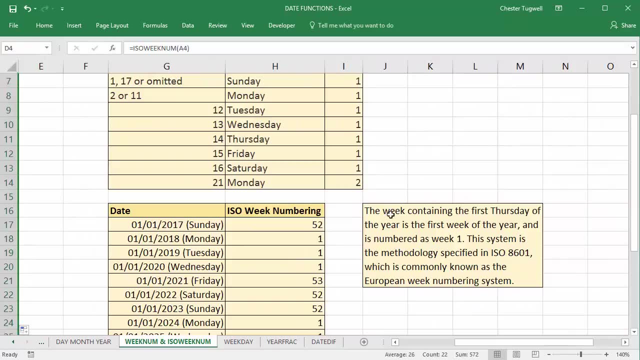 Okay. so if I give a date here, you can see that these answers correspond to these answers here. So week number 21, using weeknum, is the same as ISO weeknum, And let me just explain a little bit about that Now. it basically follows this rule: The week containing the first Thursday of the year is the first week of the year and is numbered as week 1.. This system is the methodology specified in ISO 8601, which is commonly known as the European week numbering system.